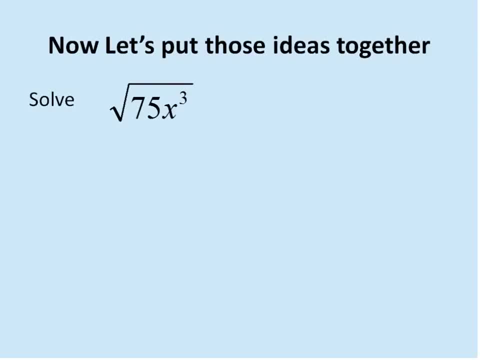 into a question involving a number and a variable. All right, So we have the square root of 75 x to the power of 3.. We're going to look at the number and the variable separately, because 75 x to the power of 3 is the same as 75 times x to the power of 3.. And remember: 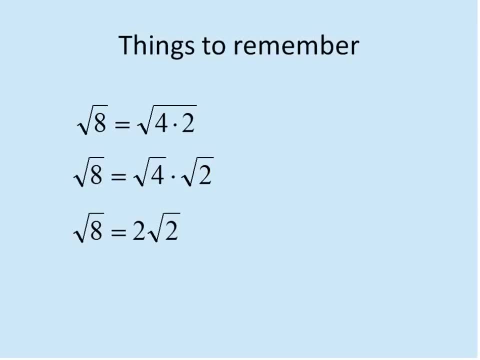 if you multiply them, you can separate them as far as square roots go. So we're just going to think about that, So we're going to think of them separately. What we're also going to do, as you see in this step here, is we're going to factor 75 as the perfect square factor of 25 times. 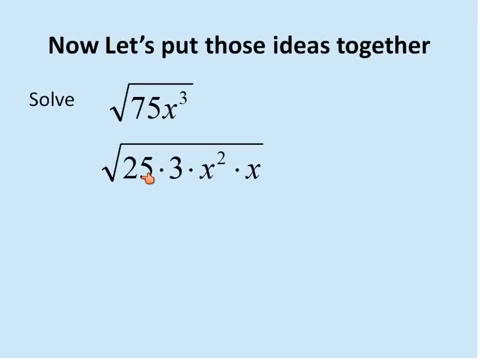 3.. 25 times 3 is 75.. 25 is our perfect square. We also know that x to the power of 3 is the same as x squared times x. And every time you get a variable, remember the square root. 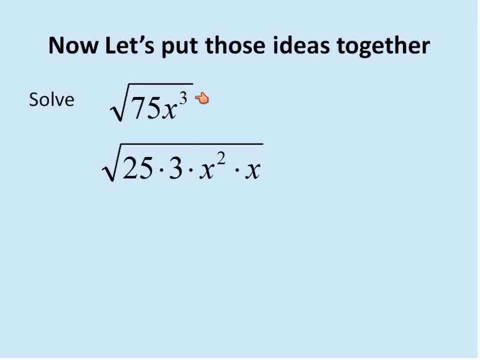 of a variable with an exponent. you just divide that by 2.. But if you have an odd number, what you want to do is take out an even number and then leave one left over, Just like that. And you'll see why in just a second. 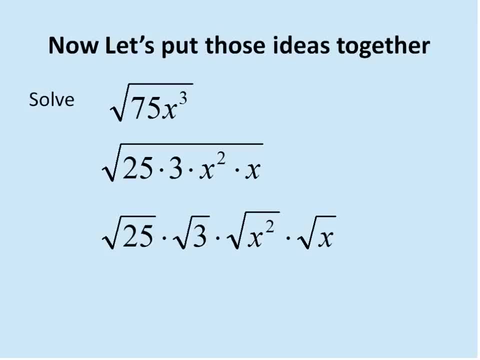 So I'm going to separate all of them using multiplication and then I'm going to take the square root of everything. that is a perfect square. So you see, here the square root of 25 is 5.. The square root of 3 remains the square root of 3.. And when I divide it by the, 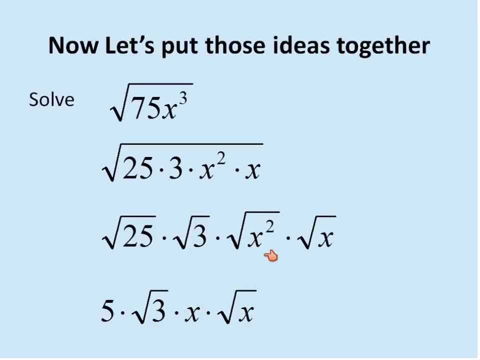 The square root of x squared becomes x. See how we can factor that one, because it's an even-numbered exponent. We just divide it by 2.. 2 divided by 2 is 1, so we end up with x to the power of 1.. 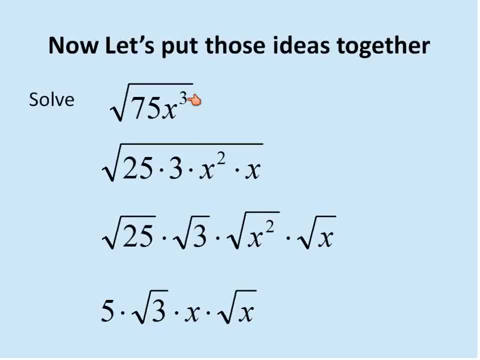 And that square root of x that's left over because we have an odd number up here, is going to remain. So in the end we're going to reorganize everything, put together everything that was solved completely or factored or square-rooted- nice and evenly. 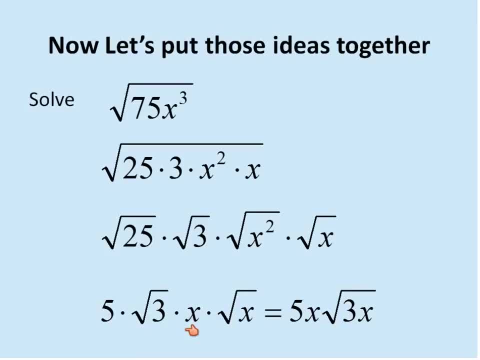 solve all the perfect squares. so we end up with 5 and x, And then whatever's left inside the square roots is 3 and x, and so that will remain inside there for our final answer of 5x times the square root of 3x. 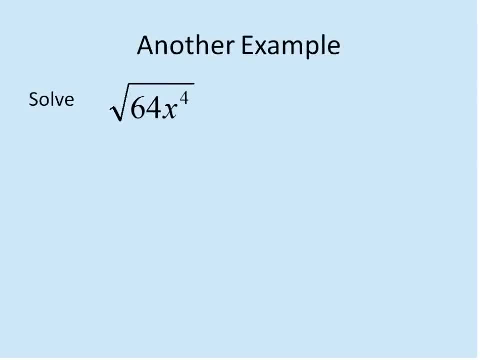 This is a challenging process. Let's go through another example a little bit more. All right, here's 64x to the power of 4.. And for this example again, I'm going to separate things into factors that are perfect squares. 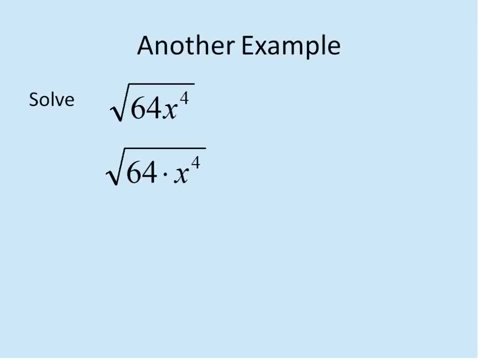 Fortunately for us, 64 is a perfect square and x to the power of 4 is also a perfect square, So we're just going to separate them like that and solve This is actually kind of a nice easy one. The square root of 64 is 8.. 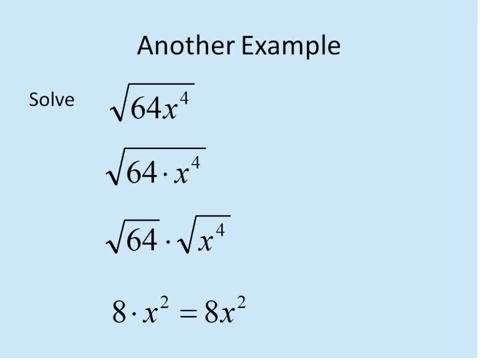 The square root of x to the power of 4 is x squared, And so our final answer is 8x squared. Notice, with this one we have no additional factors that are still under the square root symbol. Therefore, 64x to the power of 4 is a perfect square. 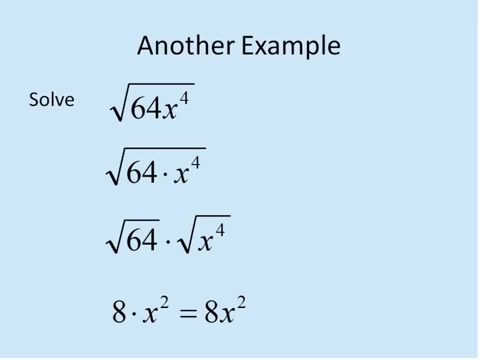 8x squared times 8x squared is a 64x to the power of 4.. All right, now our final example is going to be more like the first, a little bit more detailed, A little bit more challenging. We're going to definitely have some stuff left over under the square root symbol. 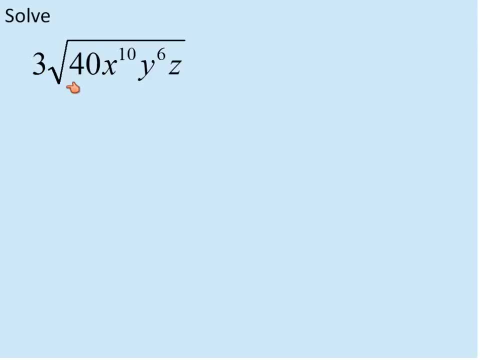 And notice, with this one I also threw a 3 out for him. That just means 3 times the square root of all of this. So in the end we'll just multiply whatever's outside the square root times 3.. It really doesn't have much of an impact. 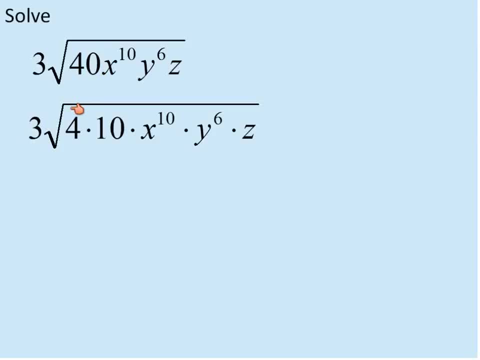 All right, we start out by again looking at our number 40. What is a perfect square factor of 40? 4.. And so we say 4 times 10.. X to the power of 10 is a perfect square because it has a nice even variable or an even exponent. 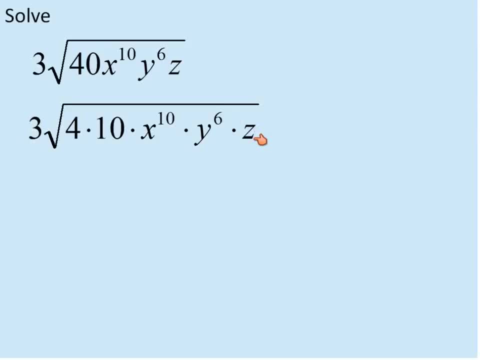 Y to the power of 6 is also a perfect square because it's an even exponent. Z, however, out here by itself is an odd number. You can't take the square root of Z and get a nice even number. 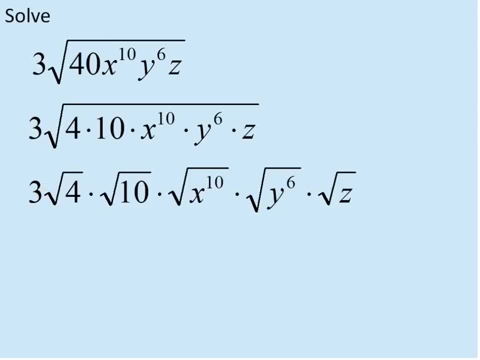 So Z is going to have to sort of remain at the end. All right, again that 3 is just staying out front. Let's go ahead and take a look at our next example. Let's go ahead and take a look at what we've done here.